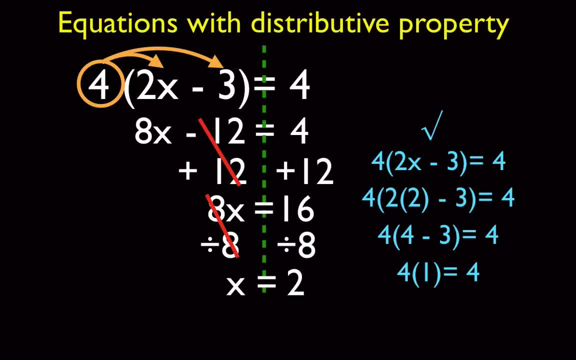 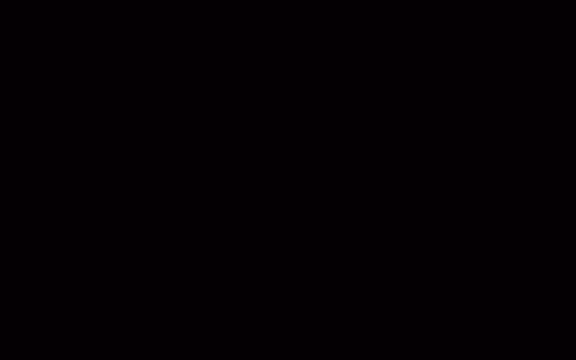 As you'll see, if we do that we get: two times two is four. four minus three is one. one times four is four. As long as that turns out accurate, then our answer is correct. Okay, so now let's go ahead and work on this one together. 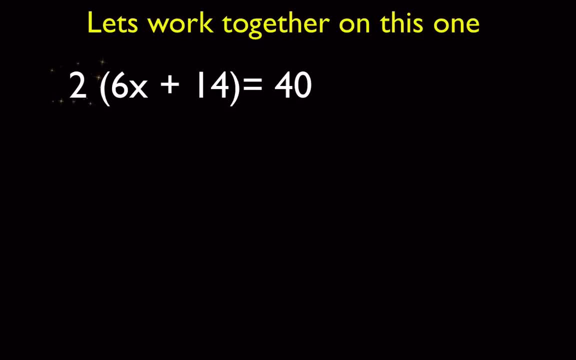 Go ahead and take that number on the outside. We're going to multiply it by both on the inside, because we notice it's a distributive property problem. Bring down the equals 40, and solve the two-step equation. You get 12x equals 12, so therefore x would equal one. 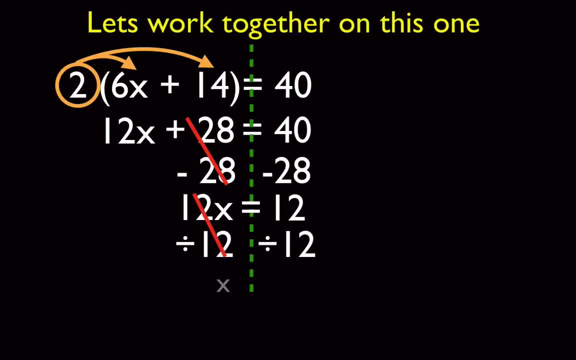 I know you might be thinking, oh, do I have to show every single one of these steps? No, I mean honestly, in Algebra 1, there's a step on your own You could probably skip here or there You could probably skip the divide by 12 step. you know just, at least on your paper. 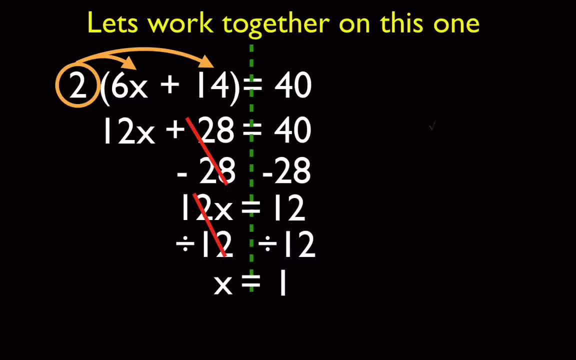 You can't skip actually doing it, but you could skip it on your paper. Checking it, I'm going to look to be sure that when I plug in that one for x, it gives me six plus four, which is 20.. Oh sorry, six plus 14,, which is 20.. 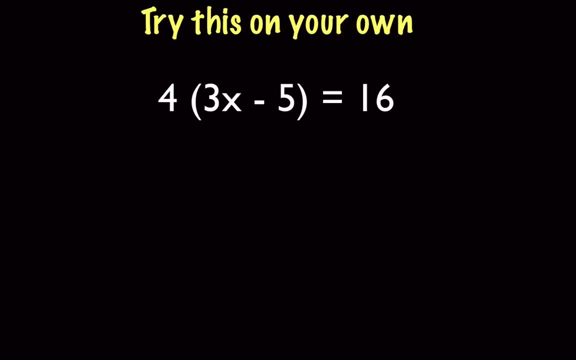 Two times 20 is 40. As long as that works, you know your answer is correct, Go ahead and try this one on. Pause the video. Take a second. When you think you have the whole answer figured out, hit play. 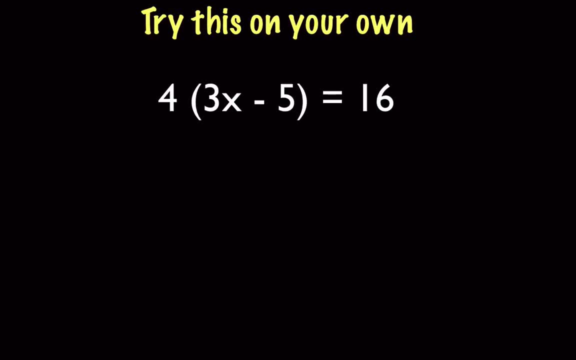 All right, so we're going to take the number on the outside, We're going to multiply it by each of the things on the inside. Okay, gives us a two-step equation which, as I've said numerous times, I hope the two-step equation is easy for you. 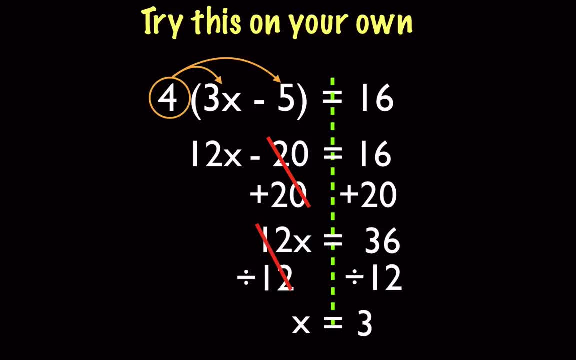 If you do it correctly, you'll end up with x equals three. Okay, go ahead and pause it again. Give this one a try as well. All right, number on the outside multiplied by both on the inside. Okay, when you get a two-step equation, all you do is you solve the two-step equation. as we already know how to do it. Okay, so we're going to take the number on the outside multiplied by both on the inside. Okay, when you get a two-step equation, all you do is you solve the two-step equation. 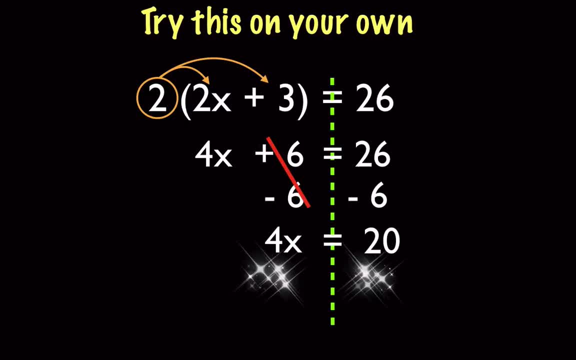 Okay, so we're going to take the number on the outside multiplied by both on the inside Should end up with: x equals five. You can check it real quickly. Two times five is ten. Ten plus three is thirteen. Two times thirteen is twenty-six. 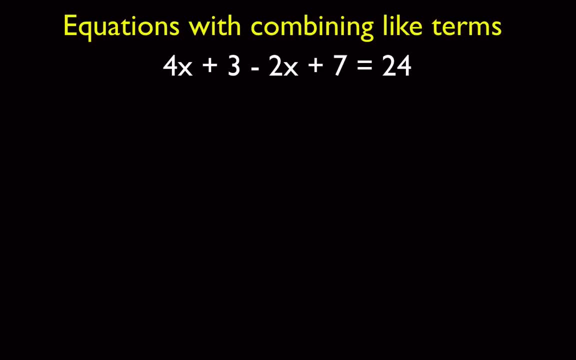 Okay. next, what we're going to do is combining, like terms, equations. So when I look at this problem, the first thing- hopefully you notice if I say hey, how is this different than a two-step equation- is we have two sets of x's and two sets of numbers. 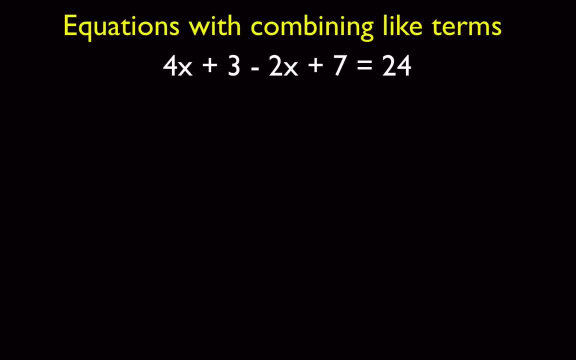 We're only supposed to have one x and one number on the left side of the equal sign, So we're going to apply what we know about combining like terms, However you choose to do it. Remember in class I showed you guys that we put the symbols. 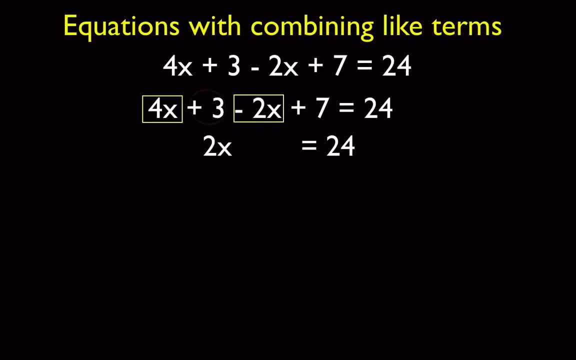 So I'm going to take the x's and put them together: 4 minus 2 is 4 minus x minus 2x is 2x And 3 plus 7 is 10. Look what we have: a two step equation. Solving the two step equation. 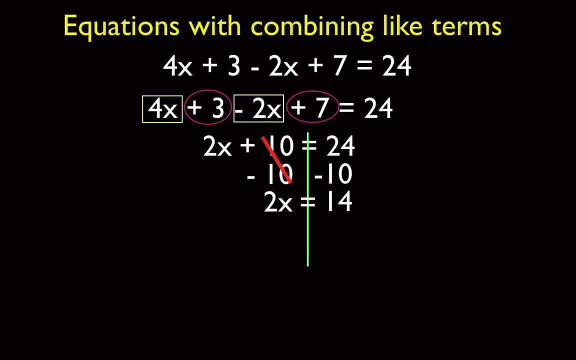 Very quickly and easily. we end up with: x equals 7. Once again, to check this answer, All we have to do is go: 4 times 7 is 28. 28 plus 3 is 31. 2 times 7 is 14, 31 minus 14. 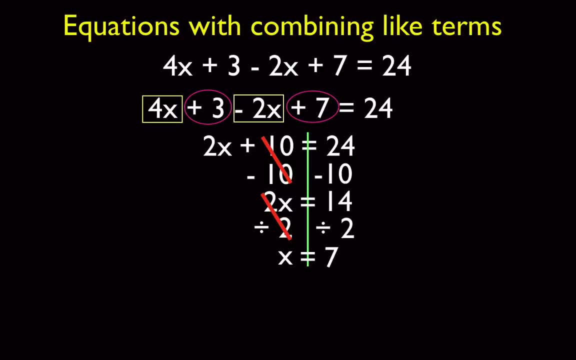 Is 17, 17 plus 7 is 24. As long as that works, you know your answer is correct. And again, this is just to show you. I know, as the problems get more complicated, The check gets more complicated as well. But with all that work involved, 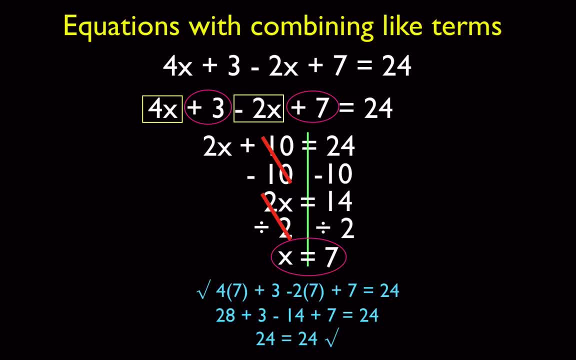 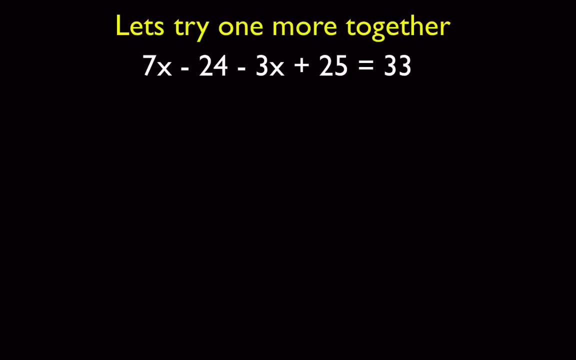 It's actually worth it, Even if you can do a mental check Or just maybe write down. Start at, Perhaps start at this step right here, Where you do the first part in your head And you get to there. Okay, let's try one more. together We're going to combine our x's. 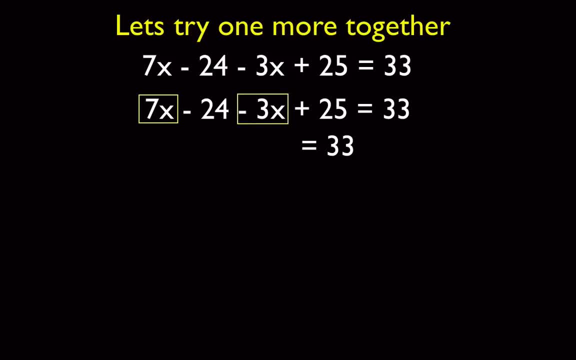 That's going to give me 4x 7 minus 3. Going to combine my numbers, 25 minus 24 is 1. Two step equation. Subtract 1 from both sides And then divide by 4, You end up with x equals 8. All we have to do from there is plug in that 8. 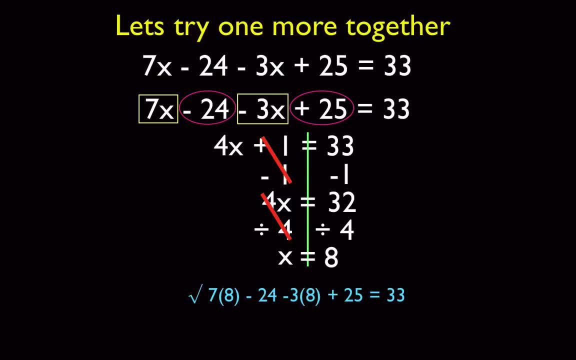 Again. I know that that looks complicated, But if you just skip to the second step, Which is 7 times 8, is 56 Minus 24 minus 24 Plus 25, You do in fact get 33, And we know for a fact that our answer is correct. 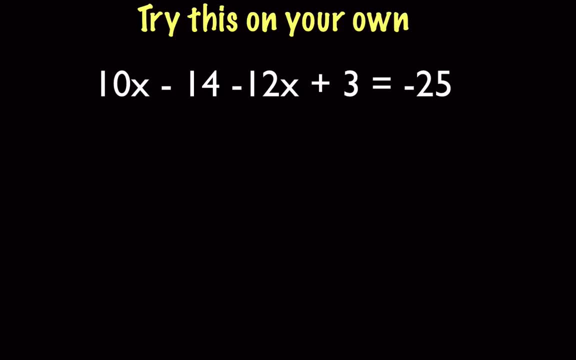 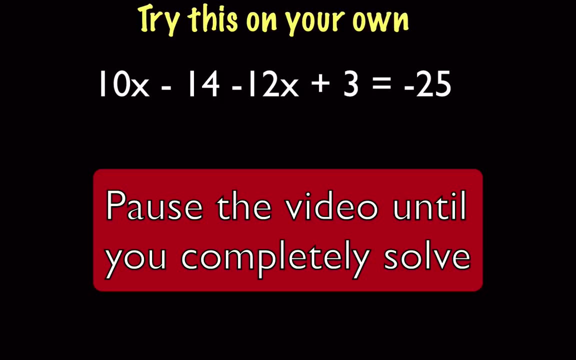 Alright, so pause the video, Give this one a try. Please do the check, if not on the paper, Then at least in your head, So you can double check that you think the answer you got is correct. Alright, so we're going to go ahead and combine those two. 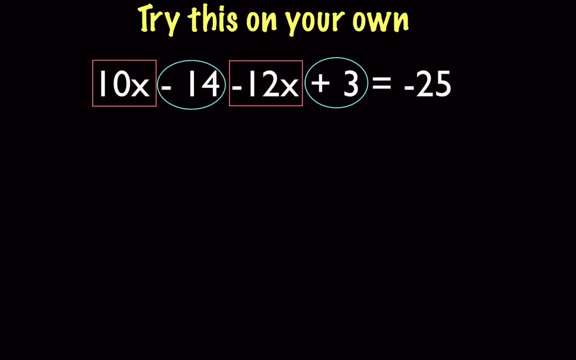 Which is going to give us negative 2x, And combine the numbers, Which is going to give us negative 11 Again. if the integer math is a problem for you, Take your time. Think of: I owe $14, I have $3, So I'm going to give it to them. 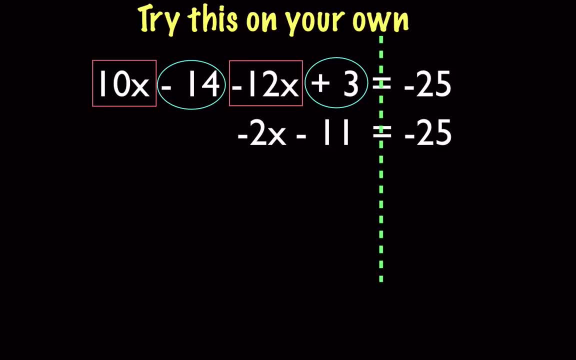 And still owe 11 Things like that. Solving with the two step equation, Dividing by negative 2 And then dividing by negative 2, I end up with x equals positive 7. Try another one on your own. Okay, 2x minus 5x is negative 3x. 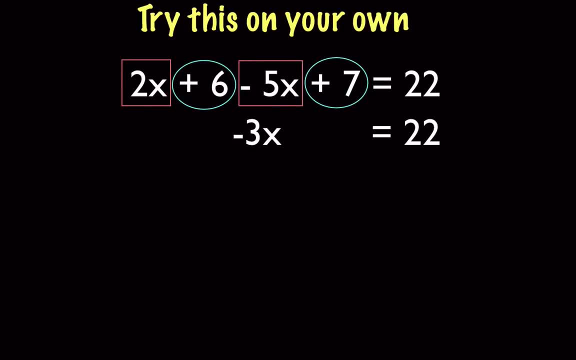 6 plus 7 is 13. Subtracting 13 from both sides, I get negative 3x equals 9. Dividing by negative 3, I get x equals negative 3. Be very careful: A 3 here instead of a negative 3 is wrong. 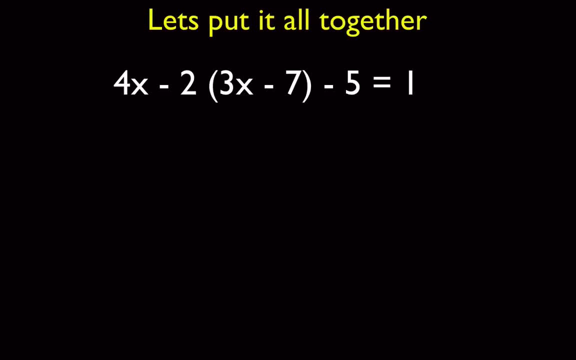 Okay, now what we're going to do is we're going to put it all together. Okay, we're going to take it one step further. What that means is, If you notice, here I have both A distributive property part And I also have a combined like terms part. 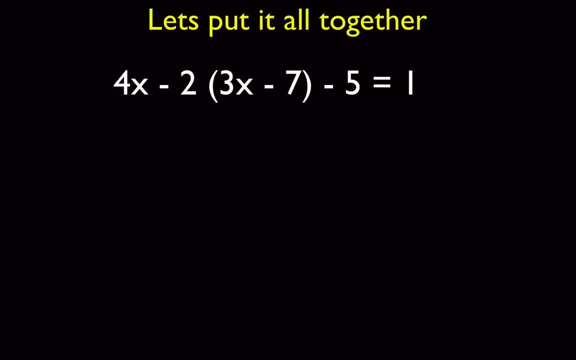 This is about the most complicated it can get. So what we're going to do now Is we're going to go ahead and start with the distributive property. Remember we did this in class for practice. You always start with distributive Circle. the negative sign included with the 2. 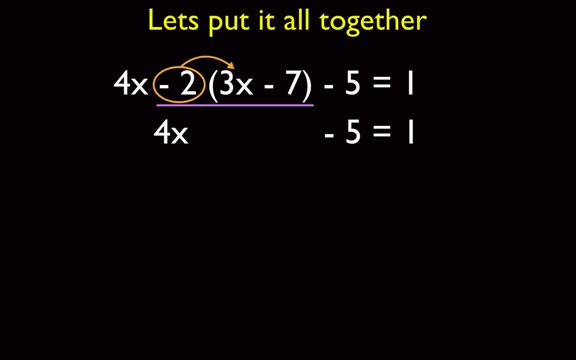 Bring down everything else. Now I multiply: Negative 2 times 3 is negative 6. Negative 2 times negative: 7 is positive 14. Now look what we have Combining like terms. I'm going to combine my x's, Which is going to give me negative 2. 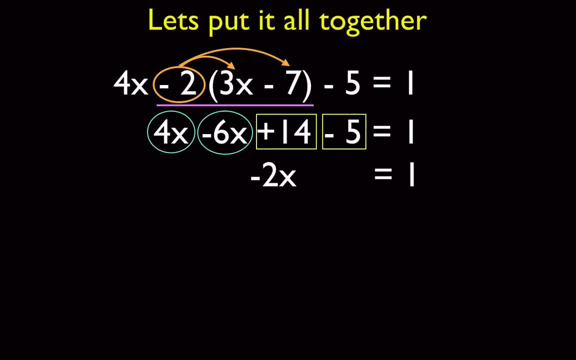 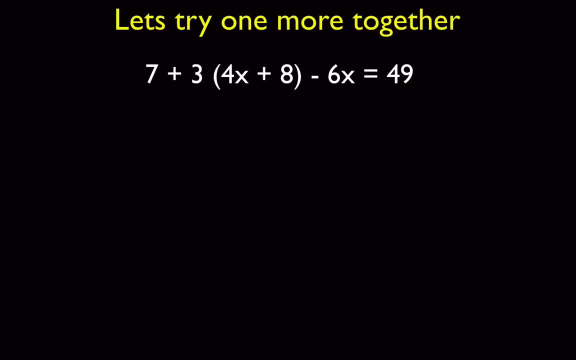 And I'm going to combine my numbers, Which is going to give me positive 9, Subtract 9 from both sides- Because look what we have A two step equation- And divide by negative 2 Gives me a positive 4. Let's try this one together Again. identify first. 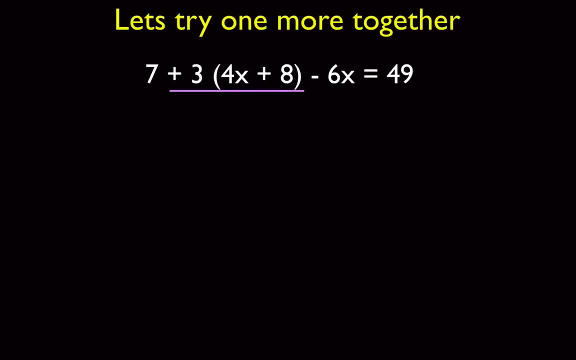 Your distributive property part. Circle the symbol outside, Including the plus sign, Even though it's a plus. Multiply, bring everything else down. Multiply the 3 times 4 And the 3 times 8. Now we combine like terms. I've got 2 sets of x's which make 6. 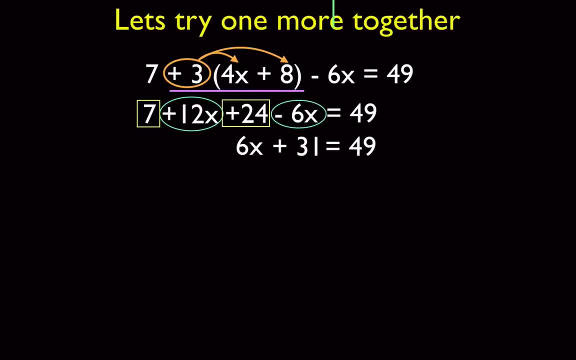 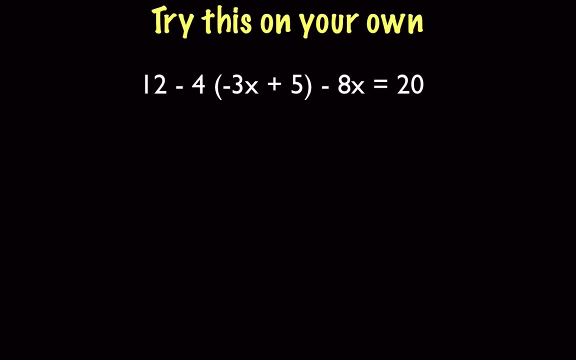 2 sets of numbers, which make 31. 2 step equation: Subtract 31 from both sides, Divide by 6 And you're set Okay. I want you to go ahead and try this one on your own. Pause the video. Alright, here we go. Start off by hopefully identifying your distributive property, part. 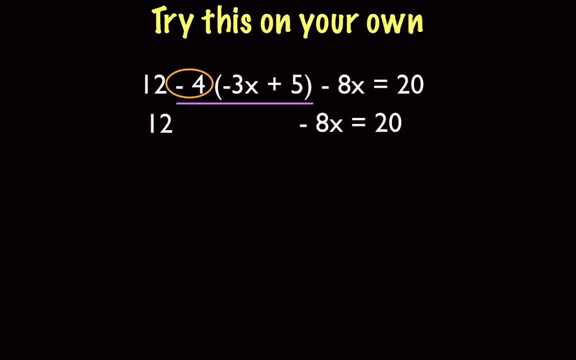 Being very careful to circle the negative sign included. So check out this step right here. Make sure you got it right. Most of you Would make a mistake right there Or Right there, Okay. so negative times- positive is negative. Negative times- negative is positive. Be very careful. Now we're going to combine like terms. 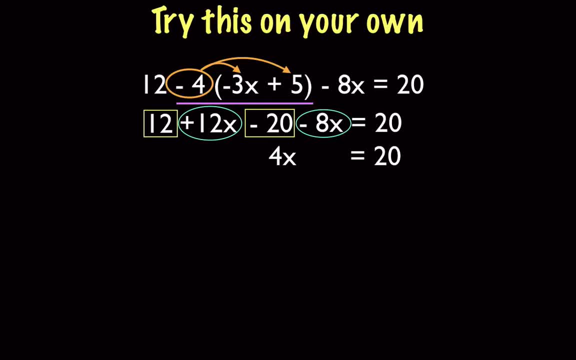 12 minus 8 is 4, And negative 20 plus 12 is negative 8. Add 8 to both sides, Divide by 4 And you get x equals 7. Okay, so what I want you guys to do now Is fill out the form down below. 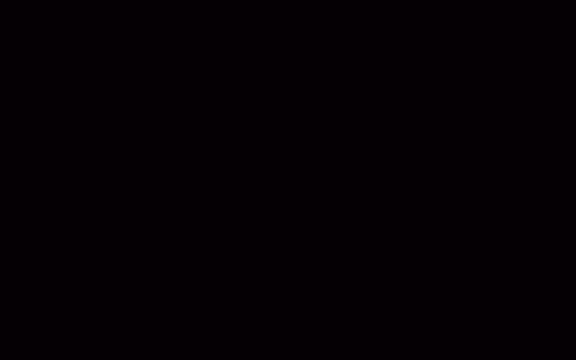 Make sure you hit submit So I can give you credit for having watched the video And then tomorrow in class We're going to go ahead and do some serious practice of this To make sure you really get it And you guys can begin getting really good at solving equations. 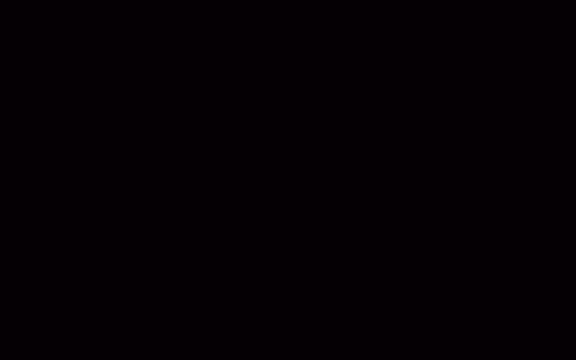 That are more than 2 steps, 3 steps, 4 steps, 5 steps. We can do as many steps as we want, As long as we remember that we want to turn that problem Into a 2 step equation. So I will see you guys soon.